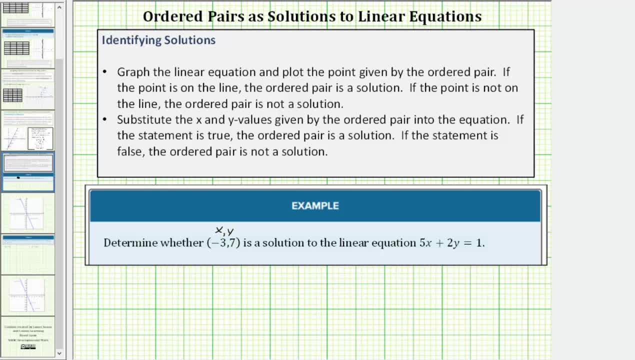 x comma y. So for this ordered pair, x equals negative three and y equals seven. So we'll substitute Negative three for x in the equation and we'll substitute seven for y. Performing the substitution, we would have five times negative three plus two times seven equals one Again. 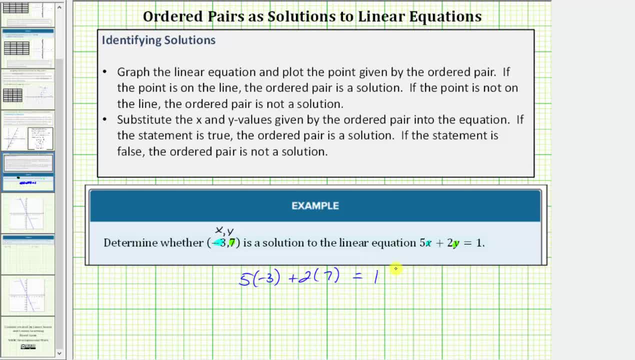 we substituted negative three for x and seven for y, And now we'll see if this equation is true or false. Five times negative three is negative. fifteen plus two times seven is equal to fourteen And negative fifteen plus 14 equals negative one, so we have negative one equals positive one, which is false negative. 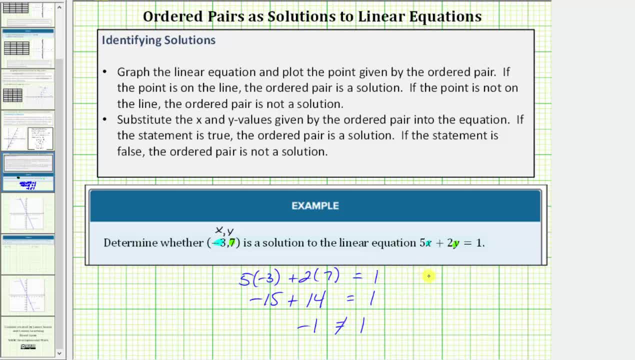 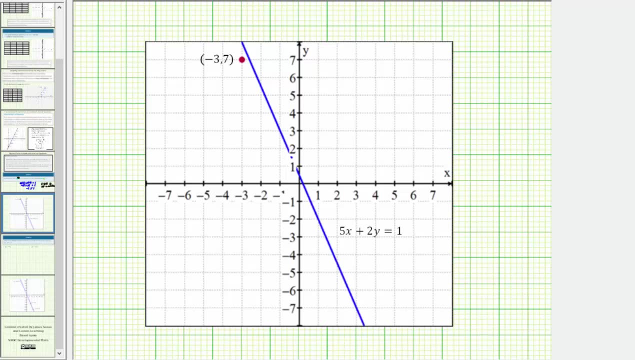 one does not equal positive one and therefore the ordered pair, negative three comma seven, is not a solution. Let's also check this graphically. The blue line is the graph of the linear equation and the point in negative three comma seven is here. 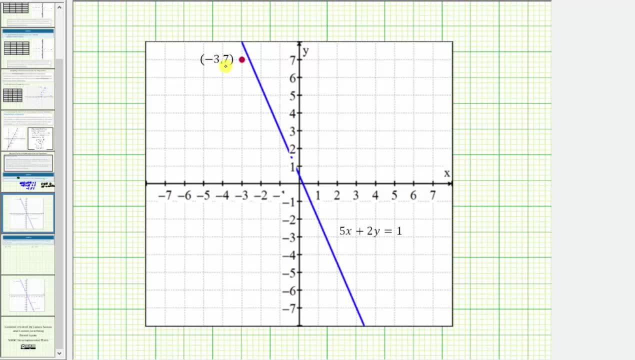 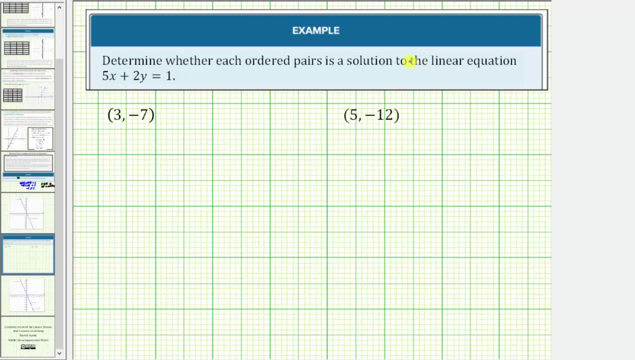 Notice how the point is not on the line and therefore the ordered pair is not a solution to the linear equation. Let's look at another example. Here we have the same linear equation and we're asked to determine if the ordered pairs are solutions. 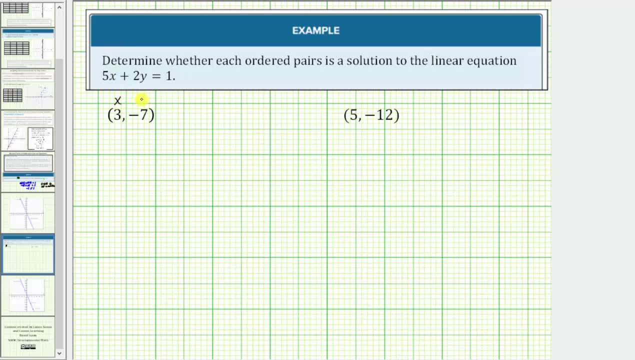 So for this first ordered pair we'll substitute positive three for x and negative seven for y. This would give us five times three plus two times negative seven. Well, five times three is fifteen plus two times negative. seven is negative fourteen and fifteen plus negative, fourteen is positive one. so we have positive. one equals positive. 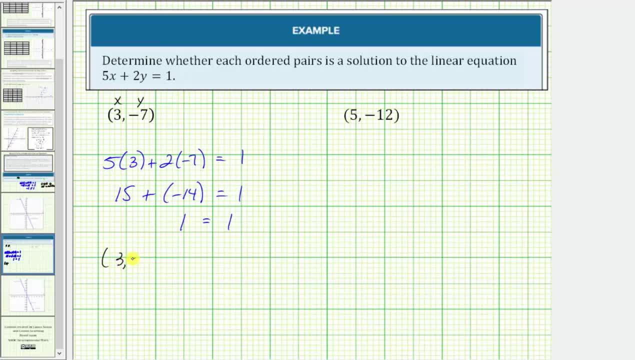 one which is true, and therefore three comma negative seven is a solution. The next ordered pair is five comma negative twelve, so we'll substitute five for x and negative twelve for y, So we'd have five times five plus two times negative twelve equals one.